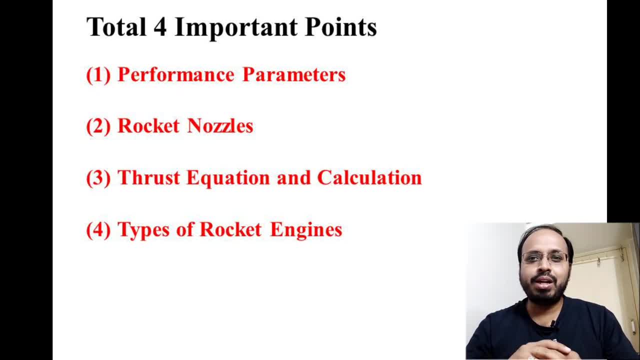 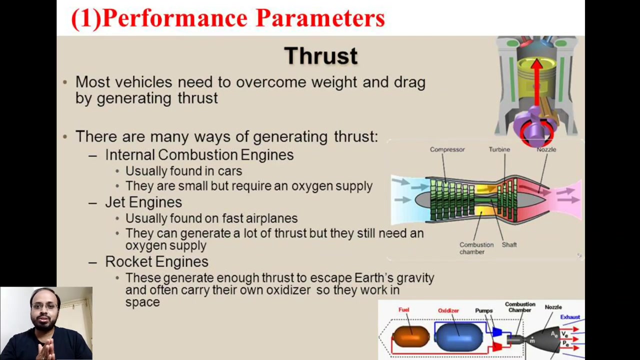 points. I have chosen to explain only the basic and fundamental of rocket propulsion So students or candidates understand or aware about that. what is rocket propulsion actually? So let us start with first important point, that is performance parameter. Performance parameter I am defining here that is thrust. Thrust is very important parameter. performance parameter of 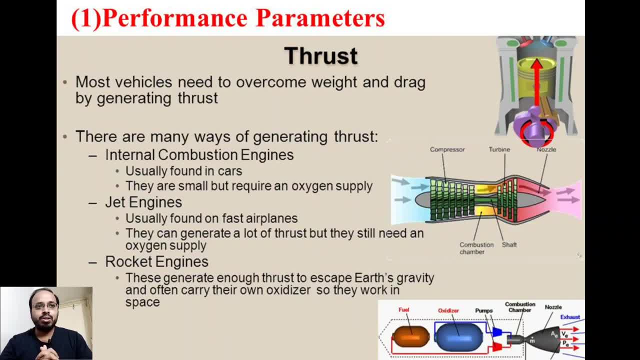 aircraft engine and rocket engine. So let us see about the first performance parameter, that is, thrust. The most value vehicles needed to overcome the weight and drag by generating the thrust. And there are so many ways of generating the thrust, That is, You can find out in different different machine like internal combustion engine, in jet engine and rocket engine. 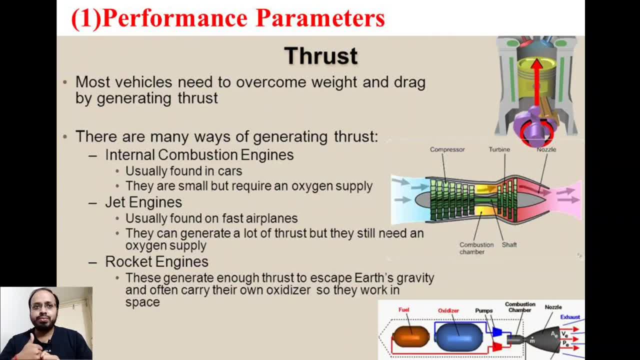 If you talk about the internal combustion engine, usually you can find out these types of engine in automobile vehicles like car buses. They are generally small in size but required oxygen supply. If you see, in the case of jet engine it is usually we are using in the aircraft, airplanes. 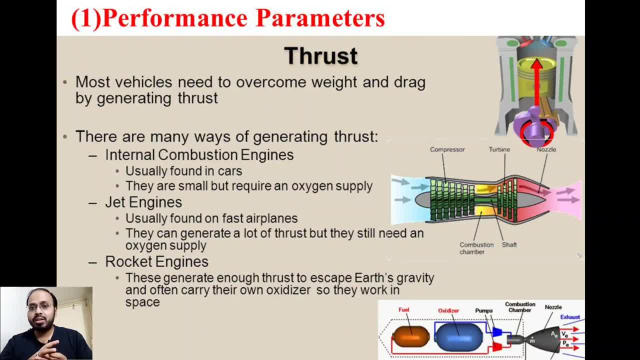 They can generate a lot of thrust, but they still needed oxygen supply, or you can say air supply. So, and in the case of rocket engine, they generated the enough thrust to escape the earth gravity And their own oxidizer, Carrying their own oxidizer. 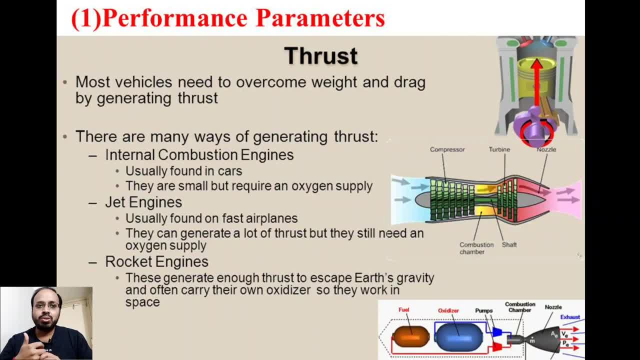 So they work in the space. So this, all three machines producing the thrust, but in different, different way. The first two category of machine, that is, internal combustion engine and jet engine, both of machine using oxygen means air directly from the atmosphere, But rocket engine carrying his own oxygen or oxidizer because it is working out of atmosphere. 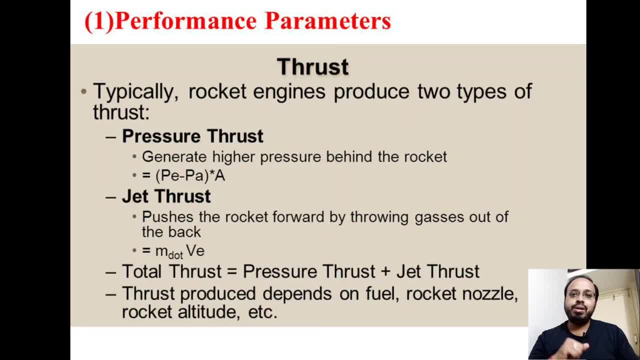 It is working in the space. That's the reason. Typically rocket engine produce two types of the thrust: The thrust pressure and second one is jet thrust. So here topic is related to rocket. That's the reason we are not going to talk about IC engine and jet engine. 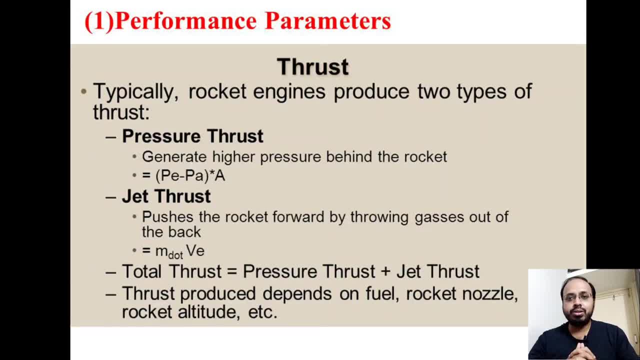 We are going to talk about only related to rocket engine. So rocket engine are able to produce two types of thrust. The first one is pressure thrust and second one is jet thrust. Pressure thrust is generated a higher pressure behind the rocket. that is PE minus PA into A. 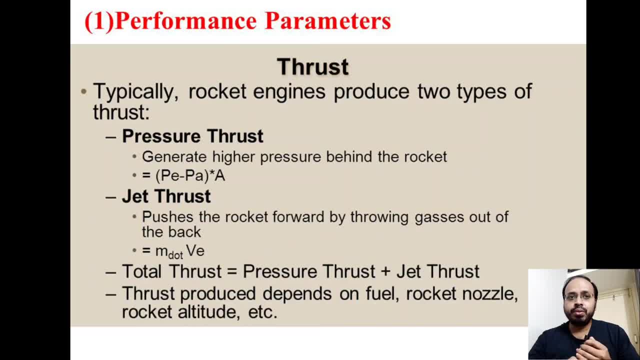 PE is the stand for exit pressure and PA is the ambient pressure of ambient pressure and A is the chamber area of the engine. rocket engine, In case of jet thrust, possess the rocket forward by throwing the gases out of the back. It is work on Newton's second law, that is, F is equal to MA mass and acceleration. 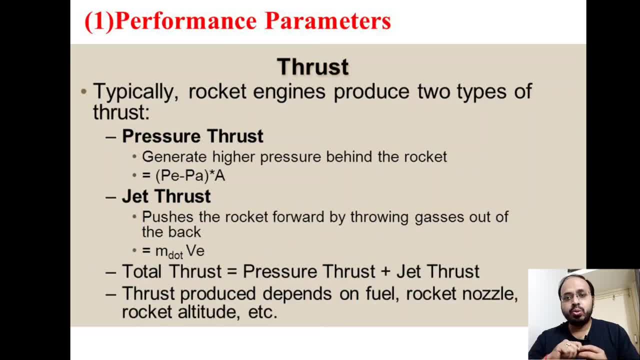 So here we are, taking the example that F is equal to total thrust, is equal to M dot into VE is that is the exist, just jet velocity, or you can say exit velocity of the jet of rocket engine. So, guys, the total thrust produced by the rocket, 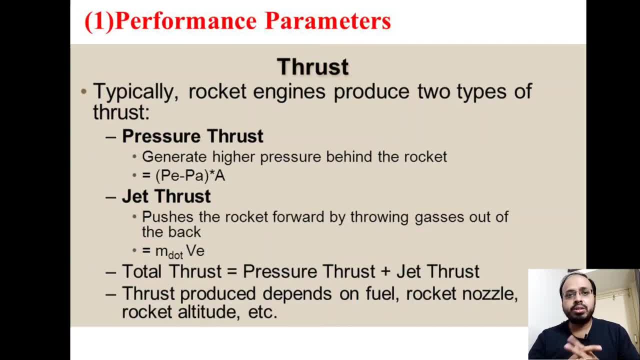 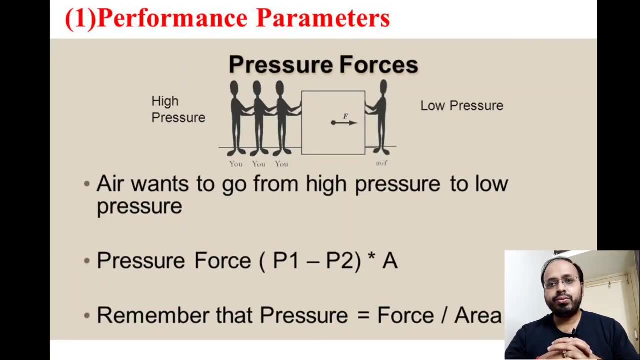 Is equal to pressure thrust plus jet thrust And jet produced by the rocket engine depends upon the few parameters. what I have mentioned in this video In earlier discussion of total thrust of the rocket engine We already seen the total thrust of the engine is equal to pressure thrust plus jet thrust. 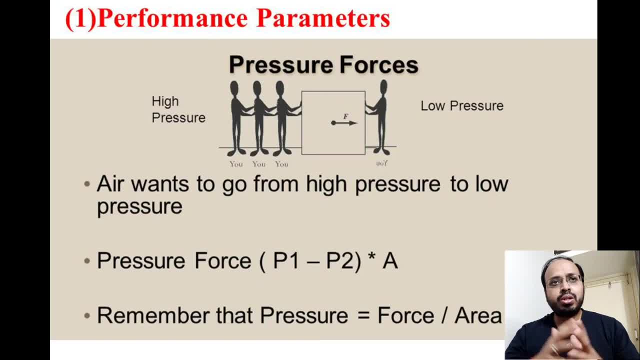 So let's see what is pressure thrust And how it is produced. The pressure thrust, or you can say pressure force- here I given the example and we know the principle also- The air or fluids wants to go from higher pressure to the lower pressure. 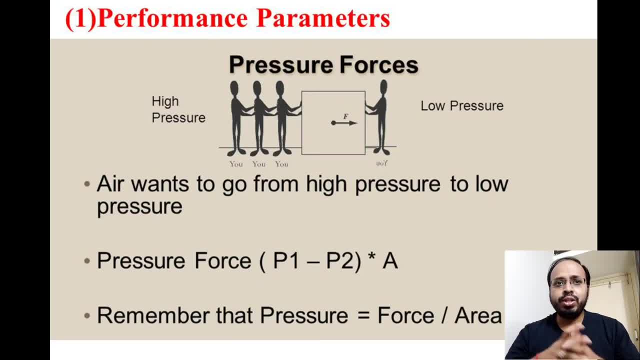 This is a general principle, everyone is know. So, with the help of this pressure, we are defining in the terms of or in the forms of: mathematically, that is P1 minus PA into A. We knows the force, we know the area And we know, also know about the pressure. 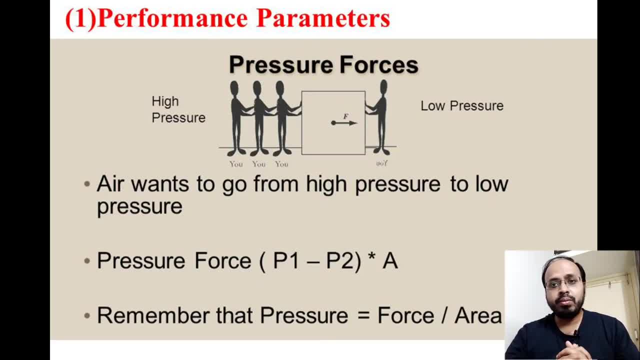 Pressure is what the pressure is force into area. So in with the help of this principle, we are defining the pressure thrust, or you can say pressure force, That is PE minus PA into AE, what we are seen in the equation of total thrust produced by the rocket engine. 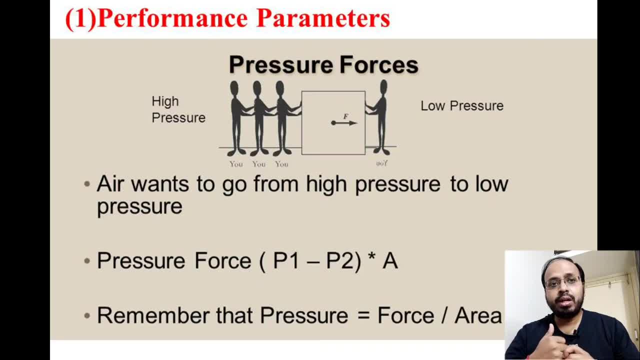 Similarly, here I have given the example that how the pressure thrust or pressure force is generated with the help of simple example. The fluid is flow from one side to another side means low energy area side, And we are writing the mathematical equations So we can easily find out that is equal to P1 minus P2 into area. 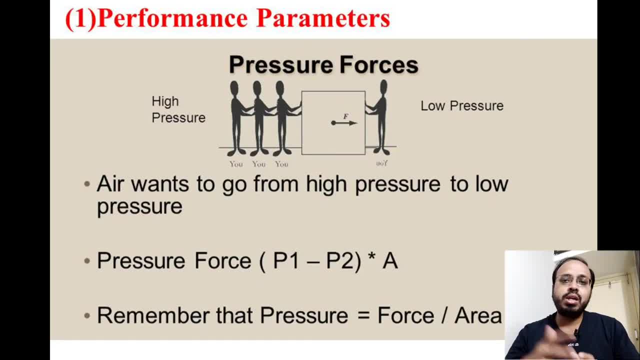 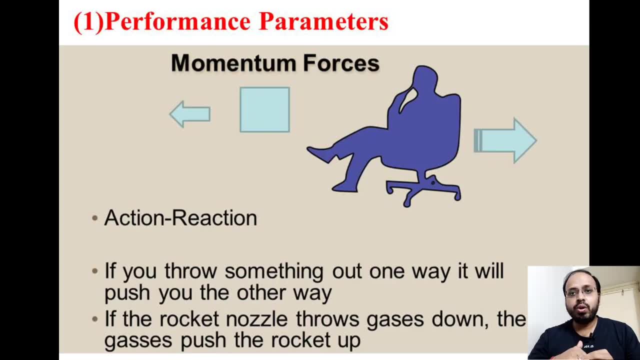 So this is about the pressure force or pressure thrust. Let's see about the jet thrust. The jet thrust is produced with the help of Newton's third law. We already know about that, And we done also discussion about the Newton's third law. 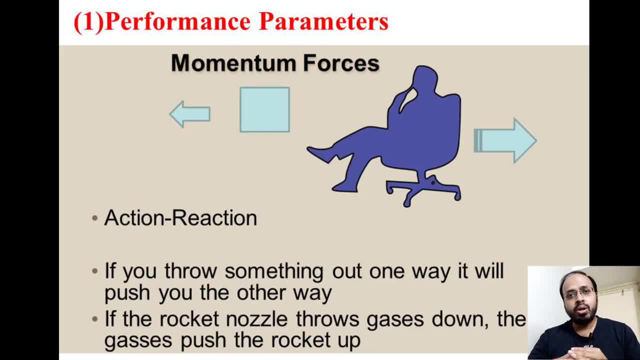 On my previous video. It's working on the principle of momentum forces. If you throw something out one way, it will push you the other way. That is Newton's third law. In with the help of that principle, rocket is working And we are defining the jet thrust, what we are seen in the total thrust formula. 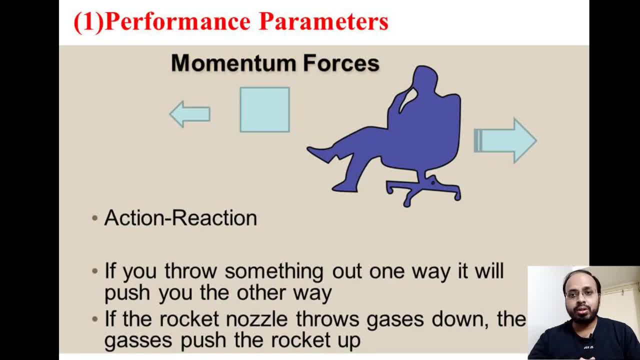 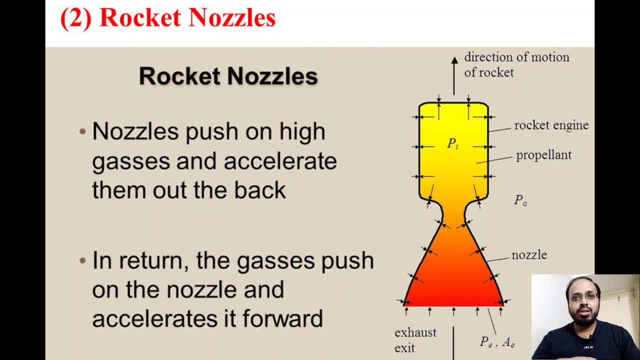 That is pressure thrust plus jet thrust, So rocket nozzle. if you see, here I given the typical picture or typical diagram of nozzle is very simple diagram. The nozzle generally push on high gases and accelerate them out the back. In return the gases pushes on the nozzle and accelerate it forward. 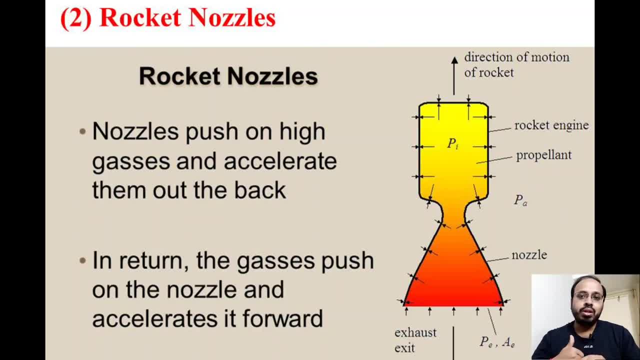 So, in the simple language, it's work similar like jet engine. Only difference is that The rocket engine carry is own oxygen or own oxidizer inside the engine And it's work on the same principle, that is, Newton's law, And producing the thrust accordingly. 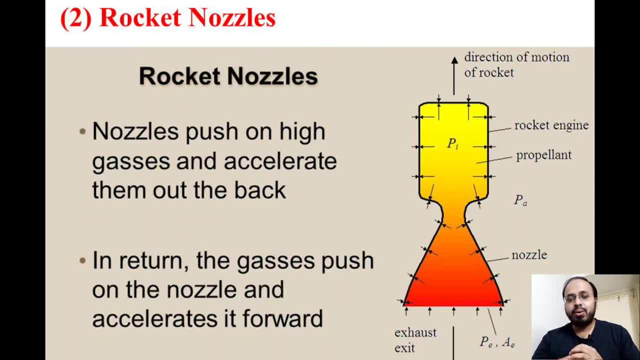 But the role of the rocket nozzle is very important Because, whatever the velocity of the exhaust gas of the nozzle is very high speed as compared to the jet engine. That's the reason the design of the rocket nozzle is very important And that's the reason we are discussing here. 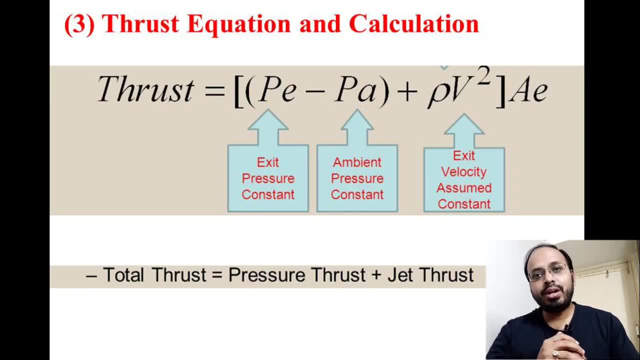 The third point is thrust equation and calculation. Here I mention the calculation also Because I want to show you the simple calculation of thrust of rocket engine. So let's see first thrust equation. Thrust equation: I already told you, the total thrust is equal to pressure thrust plus jet thrust. 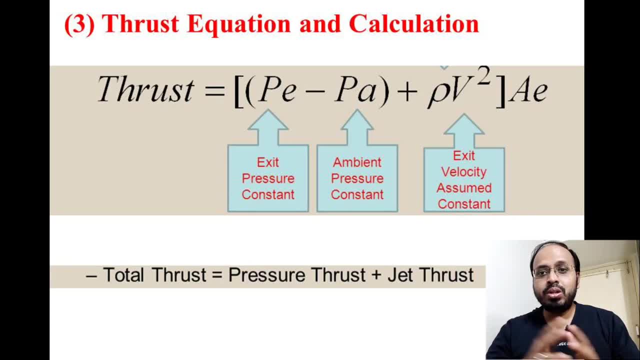 So in this equation, if you see the pressure thrust, that is P e minus P a Into A e. A e is the exit area of the engine, P e is the exit pressure of the engine, of the rocket engine, And P a is the ambient pressure. 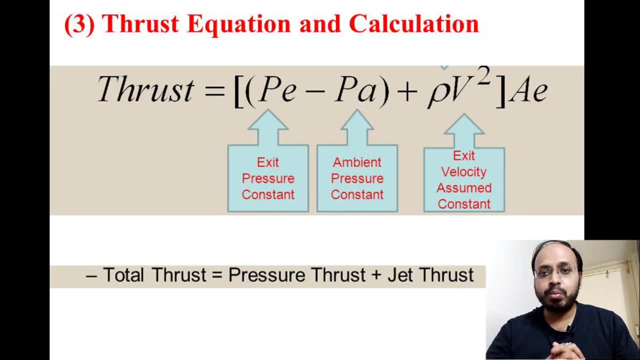 That is, you can find out in the atmosphere pressure, atmospheric pressure. So the pressure thrust that is P e minus P a into A e And the jet thrust you can see in this equation, that is rho v square into A e. So that is called jet thrust. 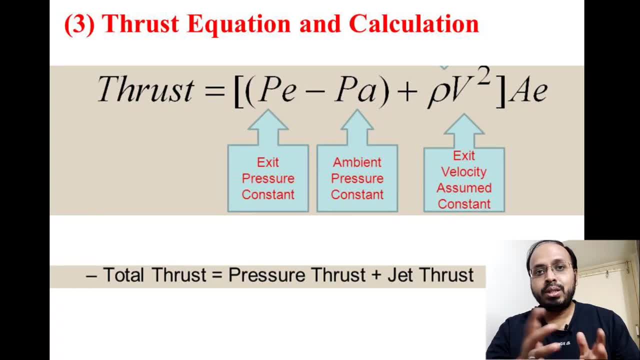 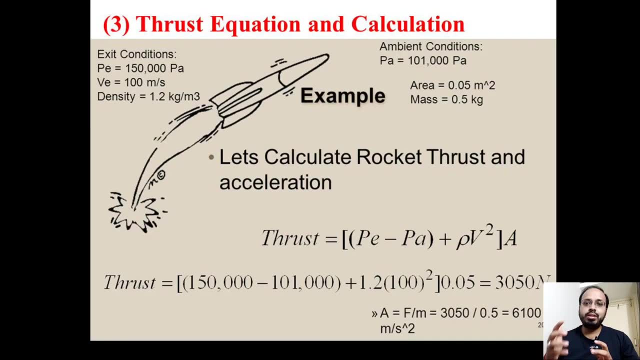 With the help of Newton's law and momentum principle. So this is the total equation, total thrust equation of rocket engine. Let's see the thrust calculation. The thrust calculation, if you see, here I have given some example- That exit condition is given and ambient condition is given. 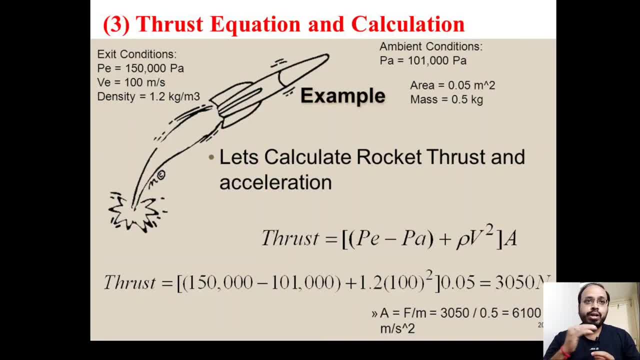 Ambient condition where the rocket engine is or rocket is flying. At that point I have taken That P? a is equal to 101 pascal kilo. pascal Area is 0.05 meter square And mass of the rocket is 0.5 kg. 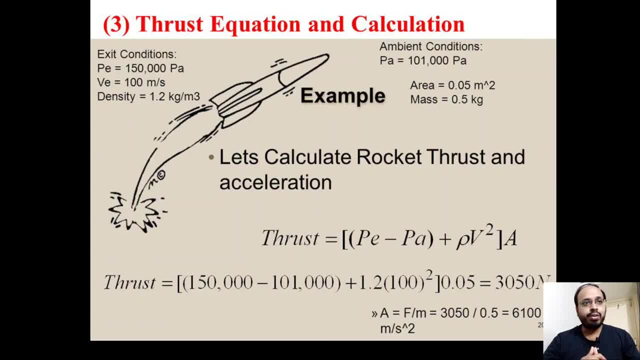 And exit condition we have taken that P e is equal to 150 kilo pascal, Or you can take in pascal also. Exit velocity of jet is 100 meter per second And density is 1.2 kg per meter cube. 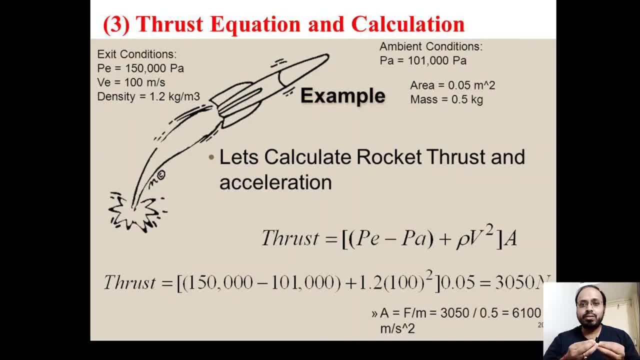 So this is a parameter I have taken In order to give some example of thrust calculation. Let's see, applying the thrust equation, what we have seen, That is, thrust is equal to P e minus P a into A e plus rho v square into A e. 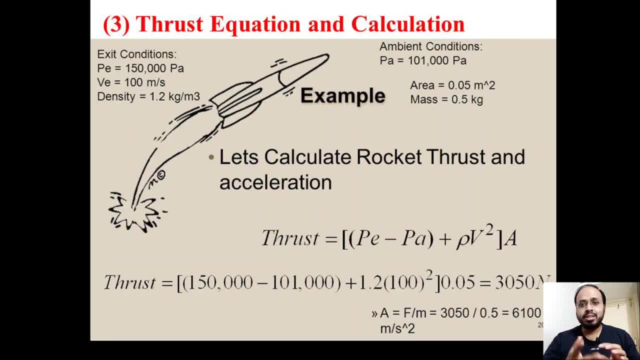 So the area is given already, Mass is given, Most of all, the parameter is given. So let's see the thrust. I am putting all the value of in the thrust equation And I got the answer is 3050 Newton. 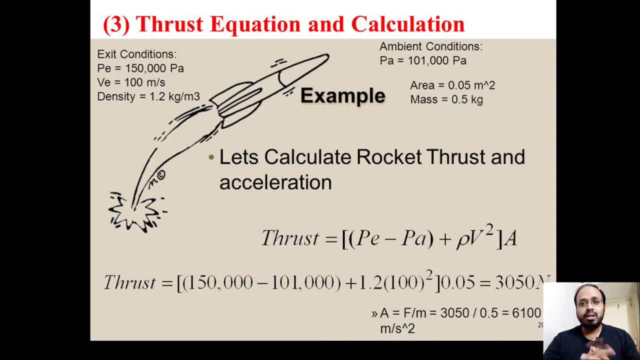 So this is a simple example: to find simple formula, to find out the thrust And suppose I want to find out acceleration. We knows Newton, second law: F is equal to m a. We already knows the mass flow rate And we already find out what is the thrust. 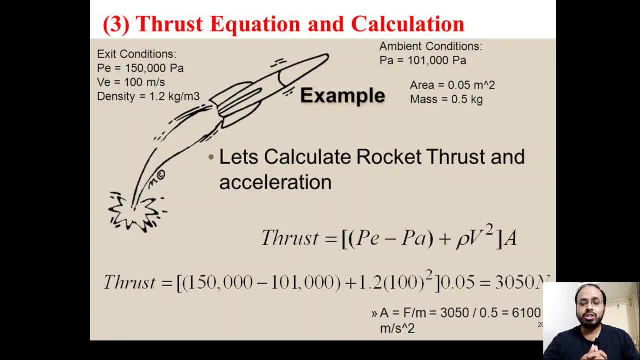 So with the help of that, you can easily find out. acceleration is equal to thrust upon mass of the rocket. So with the help of that, we can easily find out acceleration of rocket. So this is a simple basic calculation. what I need to explain to each and every candidates. 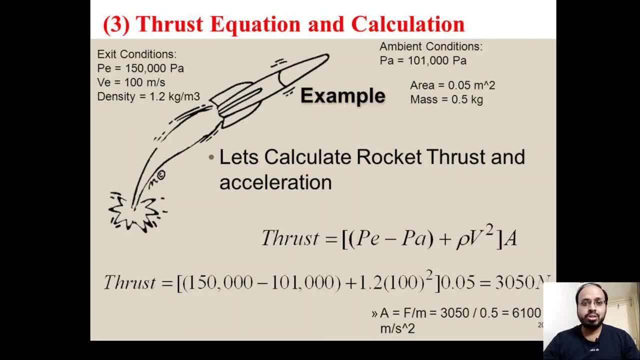 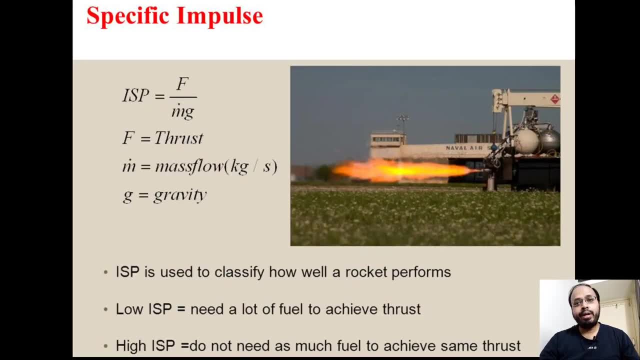 So it is very simple to find out thrust and acceleration of the rocket Before move to fourth point. First we are going to see or discuss about the specific impulse. The specific impulse is used to classify how well a rocket perform, So specific impulse is a performance parameter. 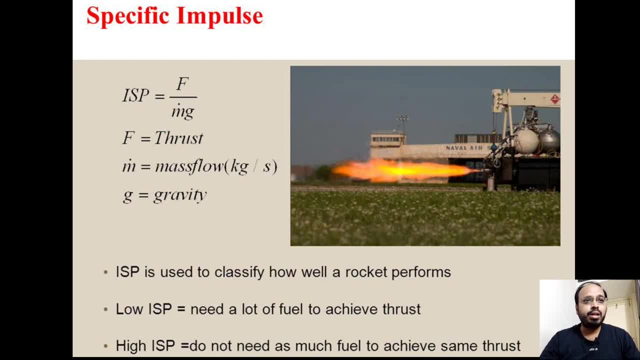 And it is defining mathematically. If you see, here I given the mathematical equation That is equal to thrust upon m dot into g Because of gravity we are taken. So this is a equation, mathematical equation of specific impulse, And specific impulse is generally defining that how the aircraft perform. 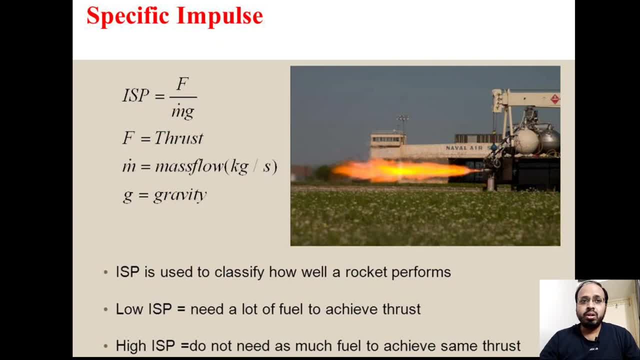 Understand If the specific impulse is low. So what is the mean? It means that need a lot of fuel to achieve the thrust, And if the specific impulse is high, it means that do not need as much as fuel to achieve the same thrust. 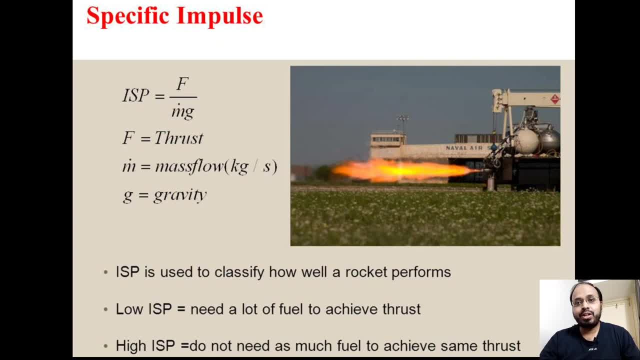 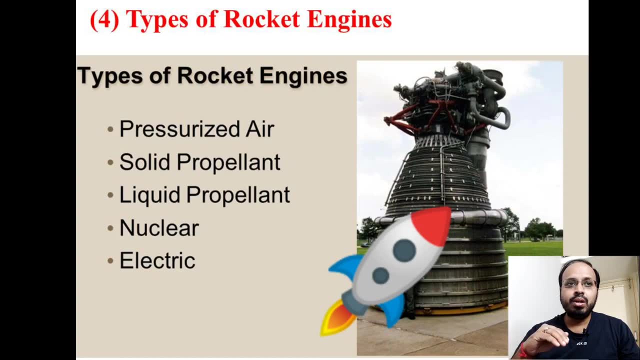 So this is the example of high specific impulse and low specific impulse. Fourth point, that is, types of rocket engine. So there are five types of the rocket engine. what I have mentioned here, That first one is pressurized air. Second one is solid propellant. 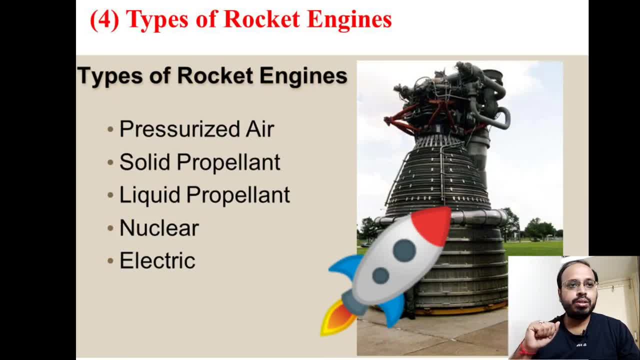 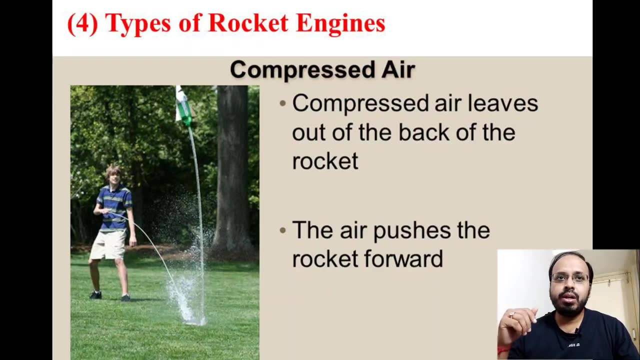 Third one is liquid propellant rocket, Fourth one is nuclear type And the fifth one is electrical type rocket engine. The first type of the rocket engine, that is compressed air. The compressed air leaves out of the back of the rocket And it pushes the air, the rocket move forward. 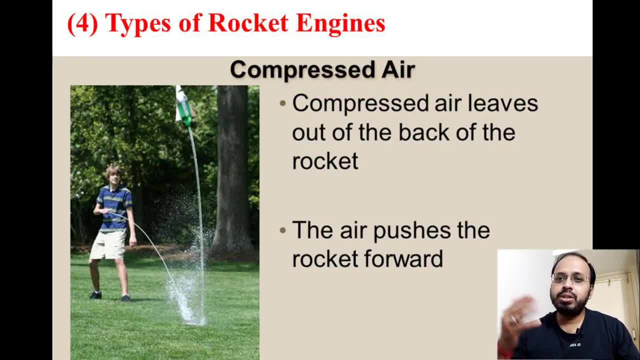 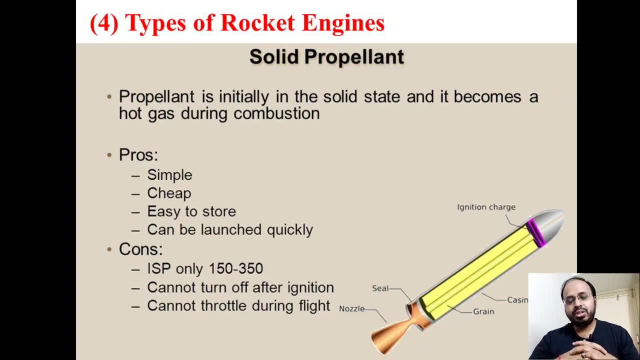 So with the help of this principle, Compressed types of rocket engine is worked. The second, solid propellant type of rocket engine. The propellant is initially in the solid state And it is become a hot gases during the combustion process in the combustion chamber. 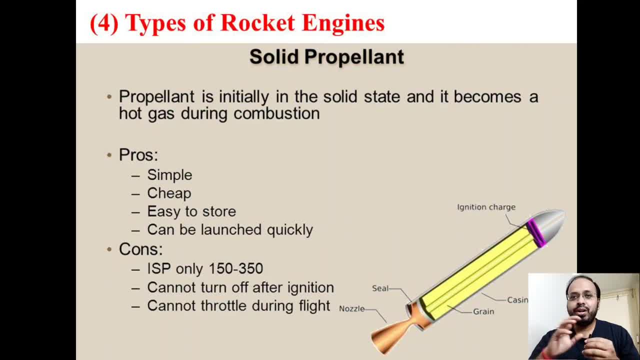 Generally, you can find out what is the advantages and disadvantages. Let us see the advantages. It is very simple in design And it is very cheap in manufacturing. also Easy to store The propellant- Solid propellant And can be launched quickly. 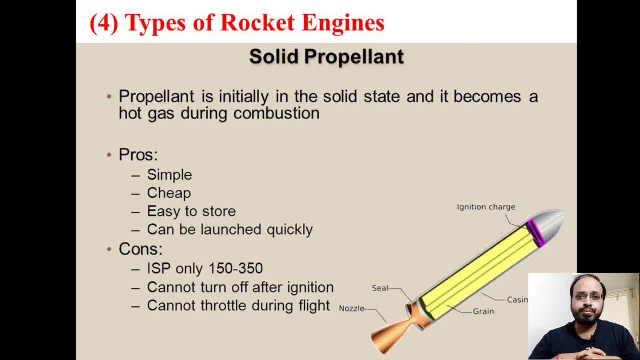 So this is the advantages of solid propellant rocket And disadvantages is that Specific impulse is only 150 to 350. Means. specific impulse is low And it cannot be turn off after the ignition Means once the ignition take place in the combustion in the rocket engine. 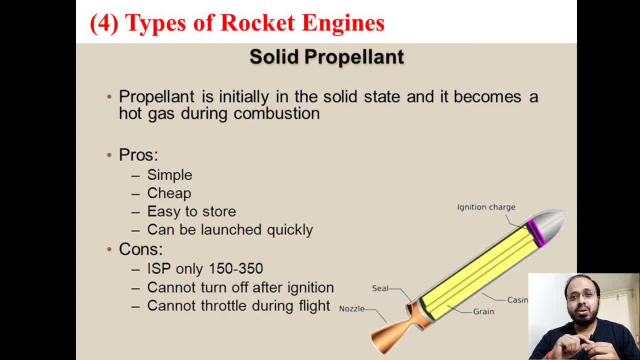 It is not going to stop And also the main drawback Or disadvantages in this engine Is that cannot throttle during the flight. So this is the advantages and disadvantages And principle of solid propellant engine rocket engine. Let us see for the liquid propellant rocket engine. 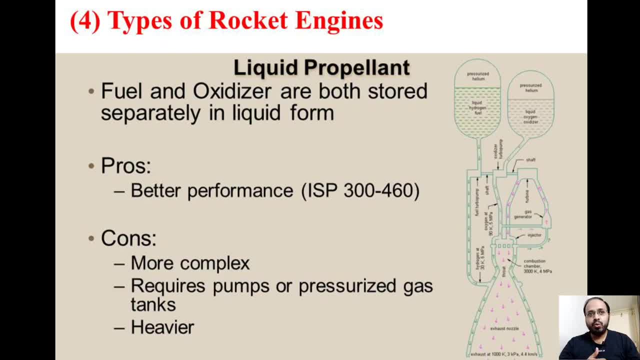 In liquid propellant rocket engine, Fuel and oxidizer are both stored separately, But in the liquid form. So this things we are doing in the Liquid propellant rocket engine And the advantages of this Liquid propellant rocket engine Is better performance. 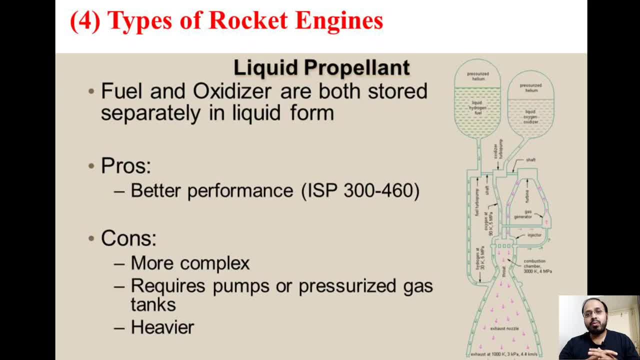 Because specific impulse is very good, Is near about 300 to 460.. And disadvantages is that It is very complex If you see The placement and storing of propellant. That is the reason is complex, So it is very complex. 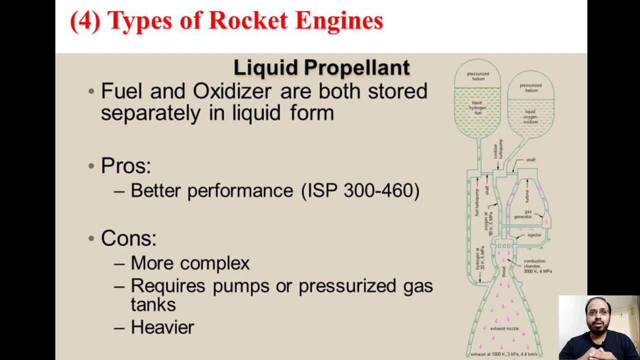 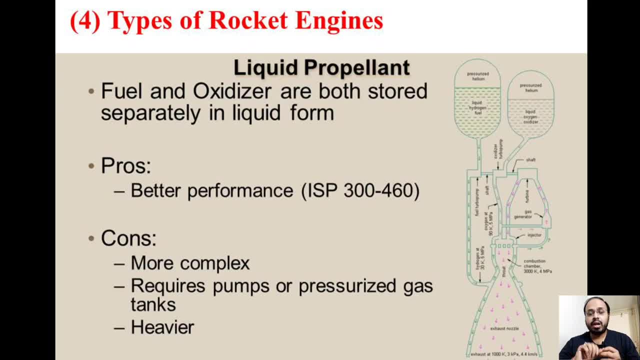 Liquid propellant Rocket engine is heavier as compared other Category of rocket engine Category of rocket engine. So this is about the liquid propellant rocket engine. So this is about the liquid propellant rocket engine For nuclear types of rocket engine. 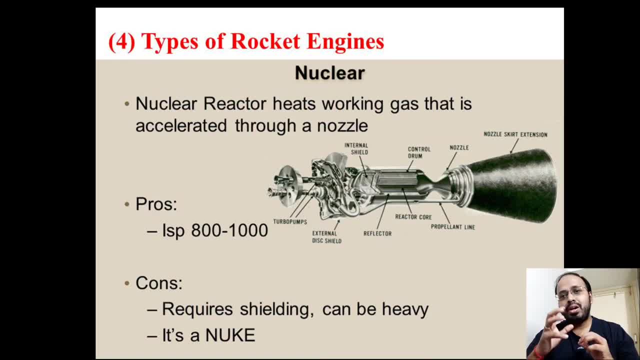 You can find out in that case That nuclear reactants heater, heats working gases, that is, accelerate through the nozzle. if you see the advantages of the nuclear type, it possess very high specific impulse, that is, 800 to 1000 specific impulse, and this advantage is that required shielding and it is very heavy because to in order to protect. 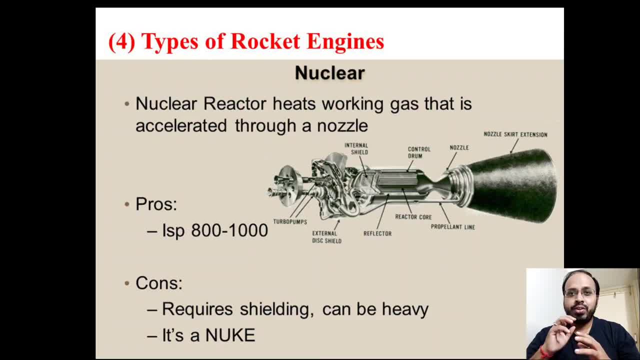 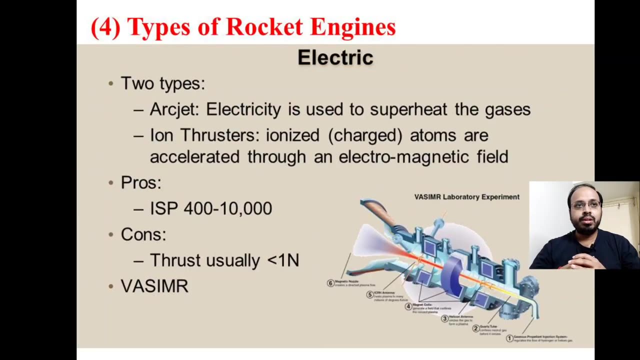 because we are using the nuclear power and guys, it is very nuke and dangerous. so this is a principle and advantages and disadvantages of nuclear type of rocket engine. let's see for electric type of rocket engine the two types of of electric rocket engine, that is, arc jet. 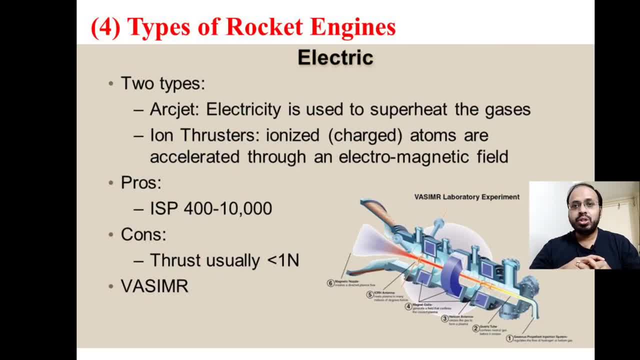 and ion thruster. the arc jet is using the electricity, electricity, electricity to super heat the gases, and ion thruster is used. ionized charge atoms are accelerate through the electromagnetic, electromagnetic field. so this is a two types of electric rocket and advantages is that it possess a high specific impulse, that is, 400 to 10,000. that is very, very high. 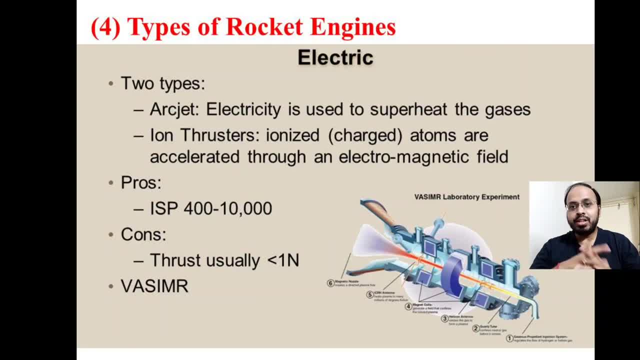 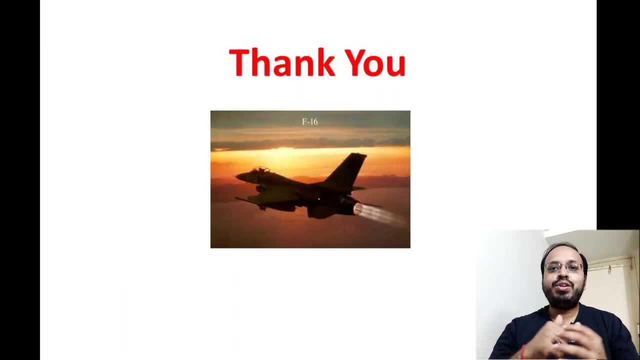 and disadvantages is thrust is usually less than one newton. so this is a two types of electric rocket and advantages is that it possess high specific Heating Zurch which isola momently bucks or burning plants. only types of electric rocket. that isyeah, this is about the ya'll contrary sais bullet, Which is that electric rocket, and advantages is THANK quarters has the strong electricity. quality of the dispenseningstars is about model readings, It is about the electric rocketтесь. So, guys, thank you for watching my video and the vacuum system. thank you for watching my video and I hope so in today topic, You ever so. in Today topic you guys are understand related to fundamental of rock in cappel We have discussed only we have to basic and goingales in from the information purposes only the pur Limited threw, cat battery toxicity At the basic and only information purposes only, overview of for rocket propulsion. So any coticidifer, a candle link, hang a free of same bit of candidates, any and other in order thende leveling field of candidates are understanding about potential on what pilots are talking about, but and only tota strong of candidates can take ¿用na O the green? 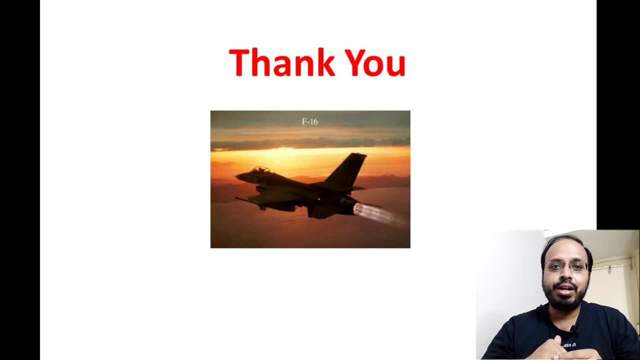 any engineering field of candidates are understand related to rocket propulsion. that's the reason i have made this video accordingly, and i have chosen all four points in order to explain related to rocket and rocket propulsion system. that's the reason i have chosen the four main points. that is performance parameter. with the help of that, i have explained.